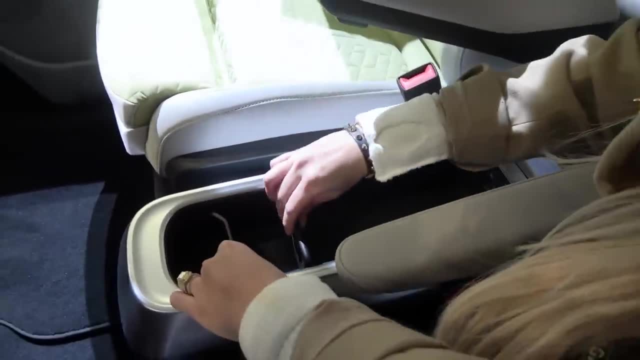 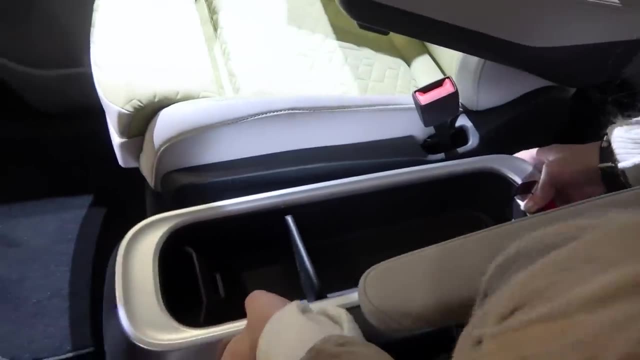 a little bottle opener here that you can slot in, and also this, which is an ice scraper, So you get all of these little things to pop in here, or you can actually remove this entire thing. There you go, Serge, My gift to you. What is that? 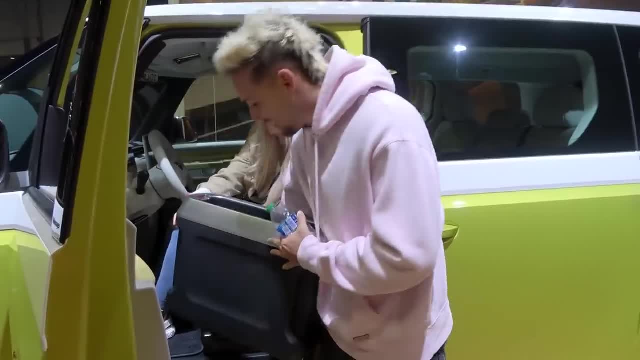 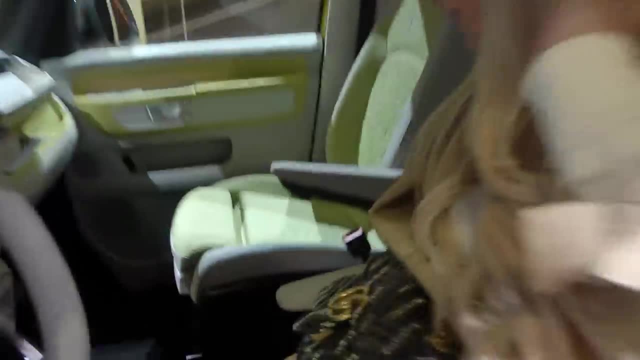 My gift to you. What's that? A center console, A center console. I've never in my life held a center console in my hands, So you can take that baby out and then here you've got all of this room for like I don't know, like an esky. if you want to put an. 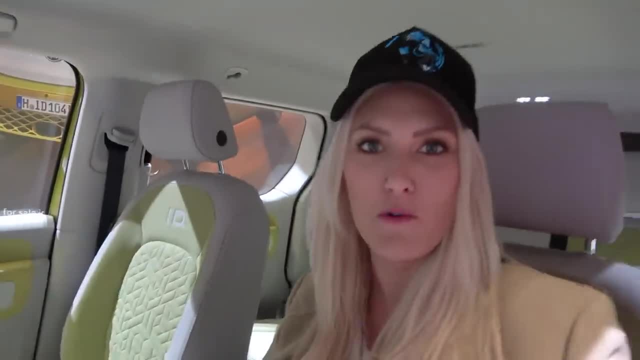 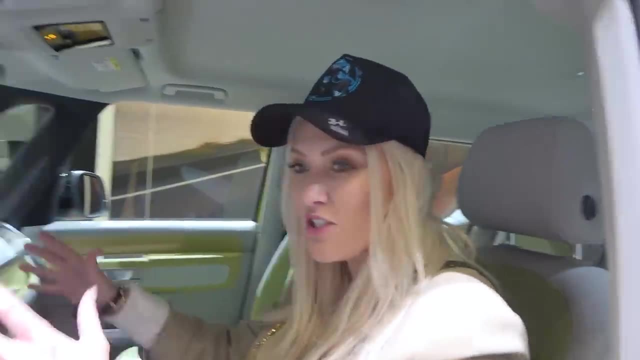 esky, or your dog, or, yes, hey, a surfboard. That's what this bus is all about, right? So they've actually changed the name from Bus to Buzz. It's fully electric. This one has just over 200. 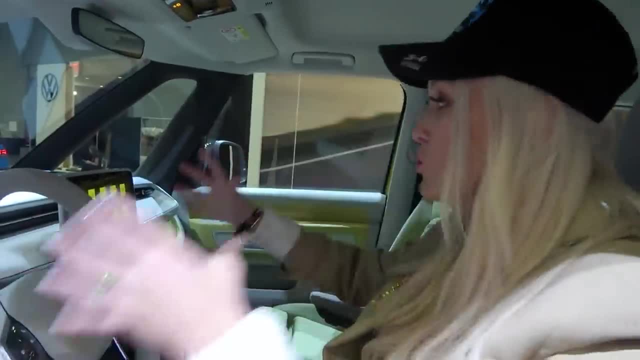 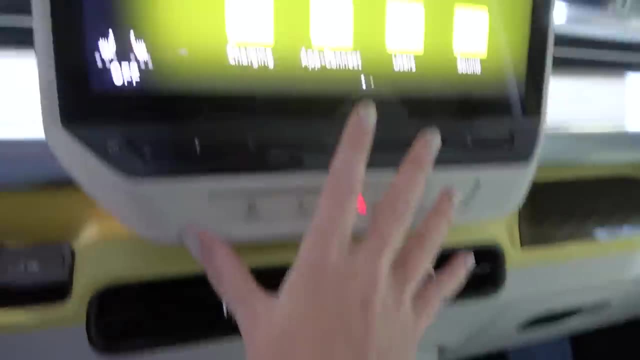 horsepower and that's what we're going to use. So it's not like we're going to release, like the range and everything a little bit later. But what I love is what you see right here is what you get. This is how it's going to look with this screen. here as well, It's all interactive. So the 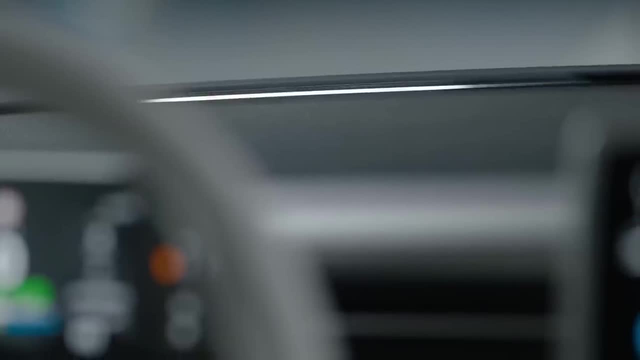 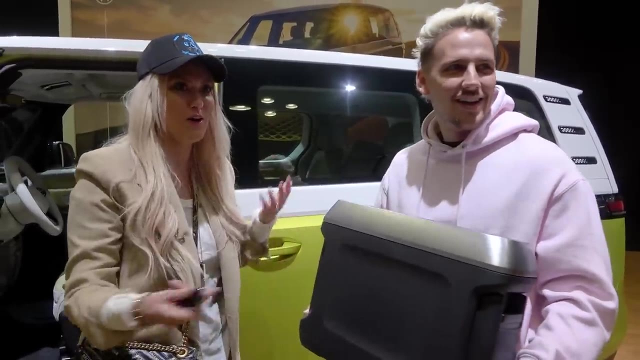 internet's a bit bad right now, but you can actually just talk to it and say, hey, ID, and it's like, yeah, what do you want, mate? Like where's the coolest surf? You know, it's like down the road, mate, Why am I holding this? Take your center console back. 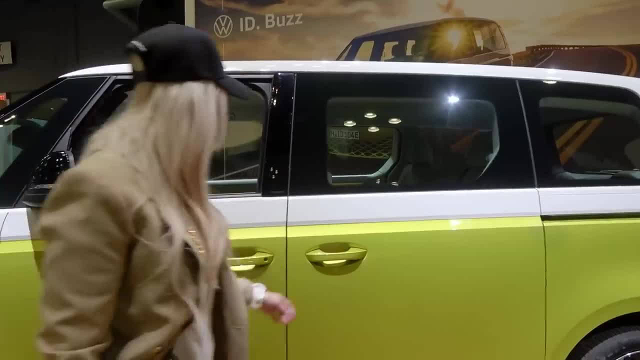 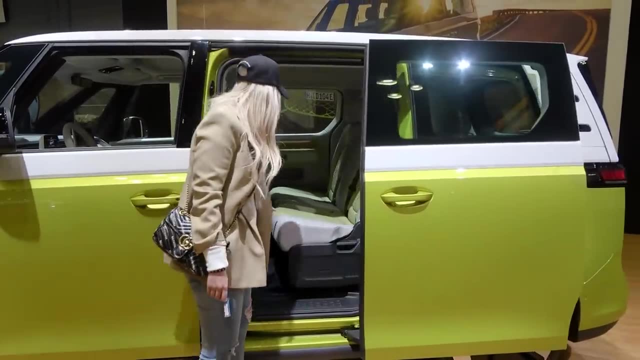 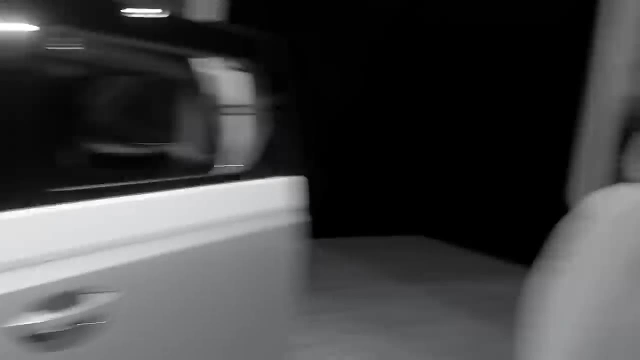 No, you can have it. That's my gift to you. I told you We'll take it to the back. Okay, squeeze this little thing in here. boom, that's how easy it is. here's your back and this fully lies down. so if you go like this, search, hold the keys. i'm holding everything right now. yeah, i'm like. 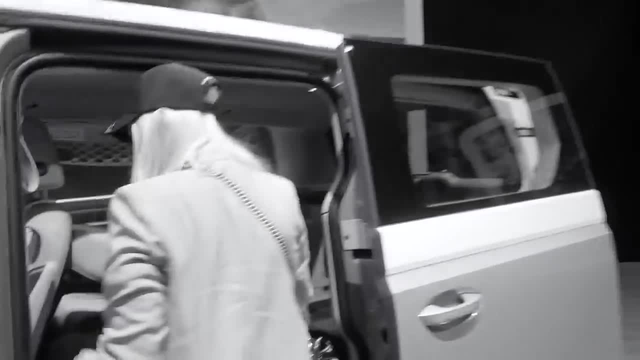 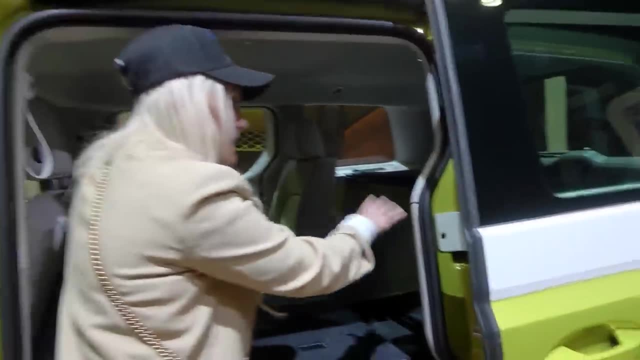 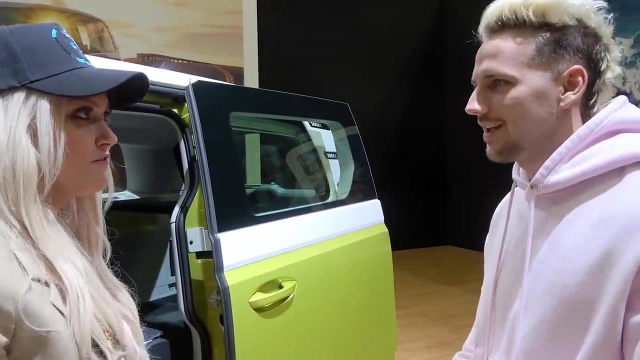 the holder- you're my assistant executive, holder of objects- put this forward. this goes down. now, what they're going to do is they're going to release an actual vw bed so you can buy a bed that fits exactly this space and turn it into like your kind of, like your home, your home, yeah, your home. 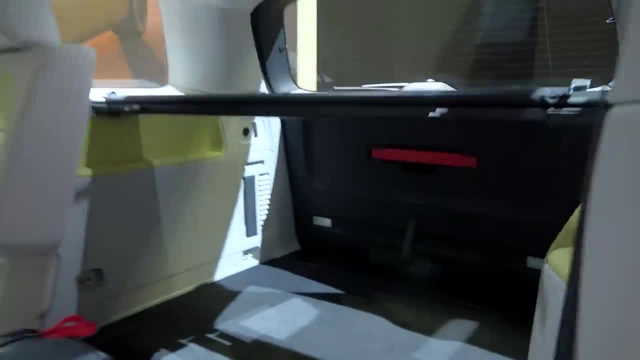 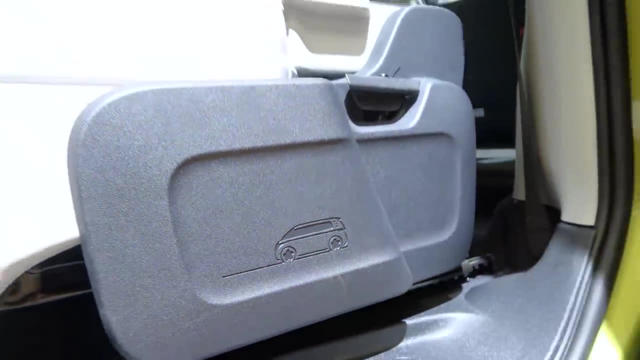 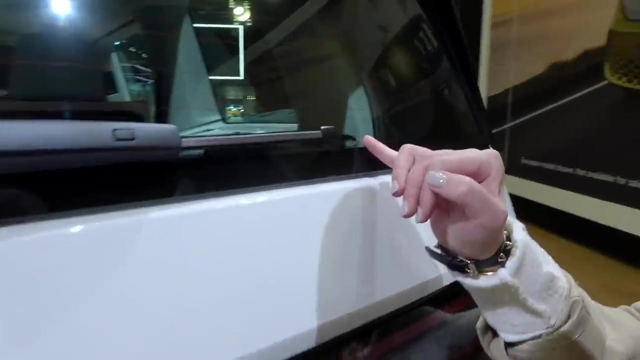 on the beach with your surfboard on the top. i like the little uh drawing on the side. yeah, so you've got all of these little like what they call easter eggs, all these little things you can discover. now talking of easter eggs, come around the back, come on, look here. you've got the little buzz, the id.